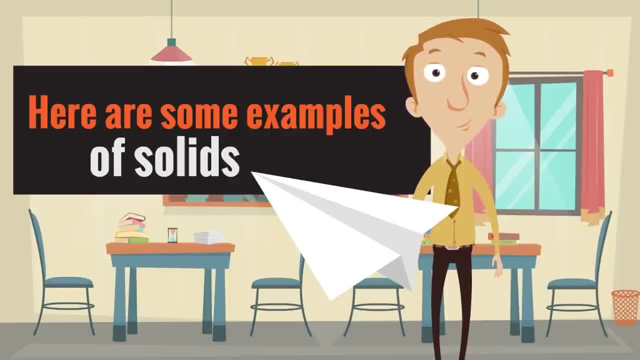 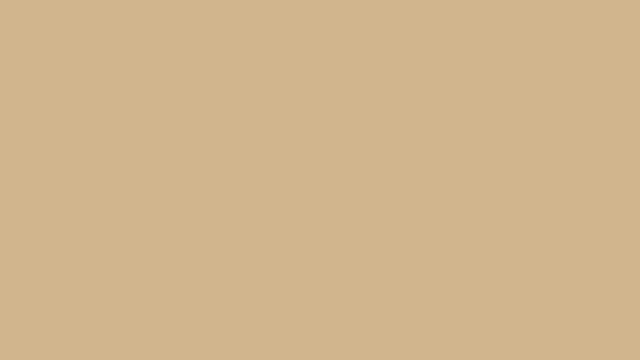 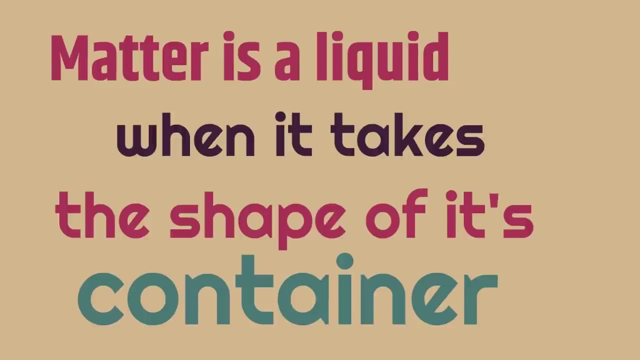 It is matter that has its own shape. It's a solid. Matter is a solid when it has its own shape. Now let's learn about liquids. Matter is a liquid when it takes the shape of its container. Here's some examples of liquids. 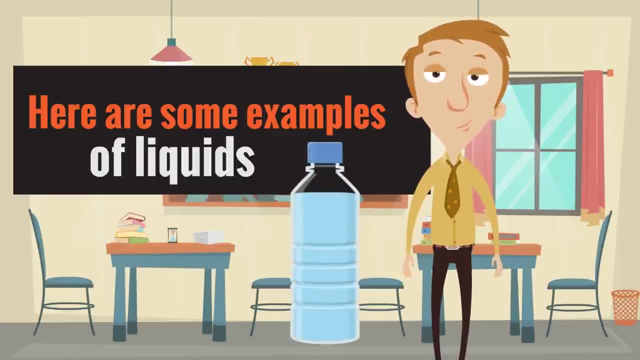 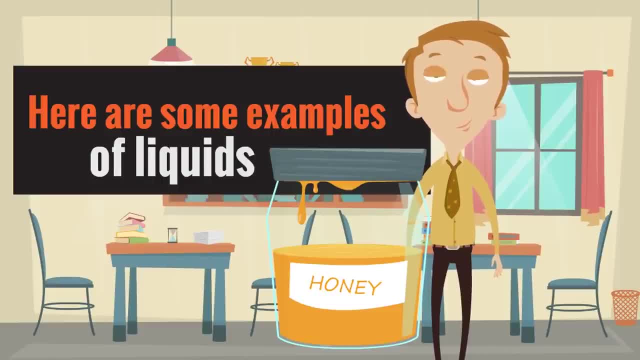 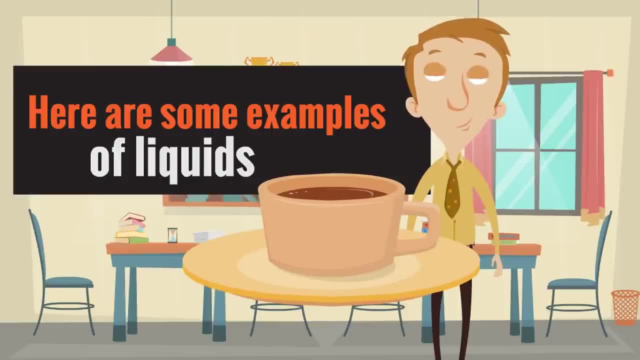 It takes the shape of its container. It doesn't have its own shape. It's a liquid. Here's the last example of a liquid: It's coffee and it's in this cup. It's taking the shape of the cup because it's a liquid. It doesn't have a shape. 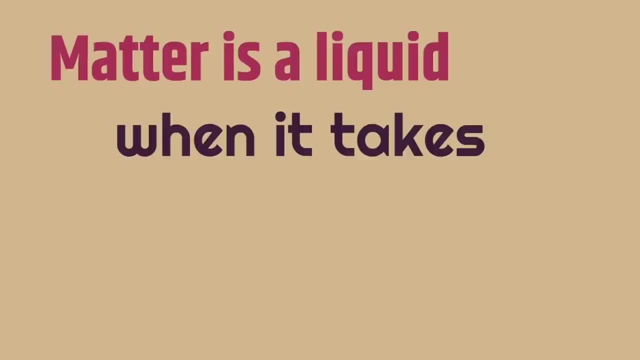 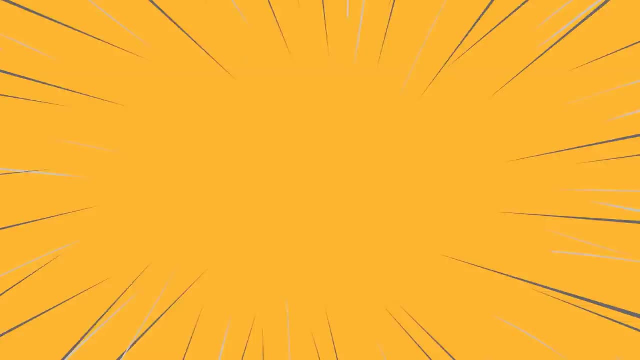 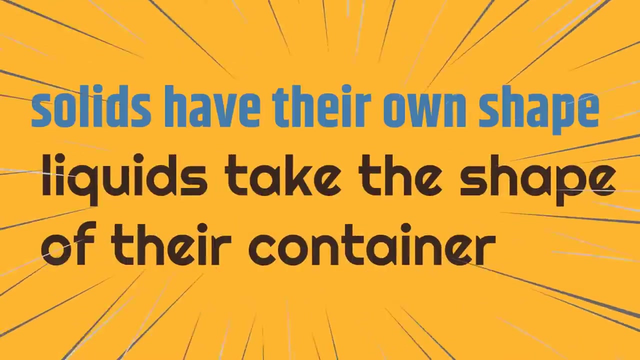 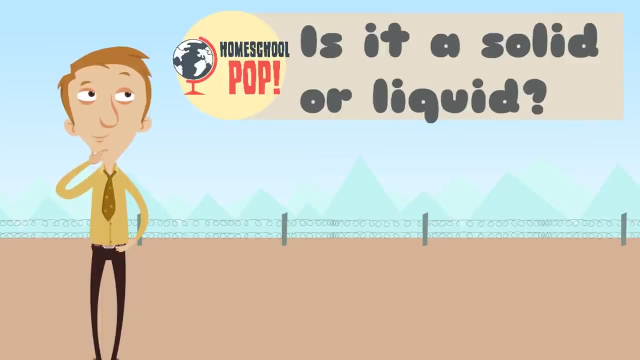 Matter is a liquid when it takes the shape of its container. Matter is a liquid when it takes the shape of its container. It's not produced, It's a cup. It's not solid, It's liquid. Slide number three: We're going to overwhelmed into uh, higher or lower a. 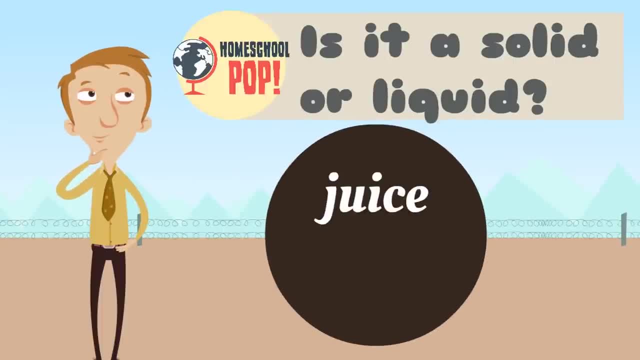 we're going to overwhelmed into uh higher or lower a. we're going to overwhelmed into uh higher or lower a recipe recipe: Add your own nonBaV��ards recipe. Add your own nonBaV��ards recipe. yeah, juice is a liquid. it takes the shape of its container. how about this? a cup is a cup.